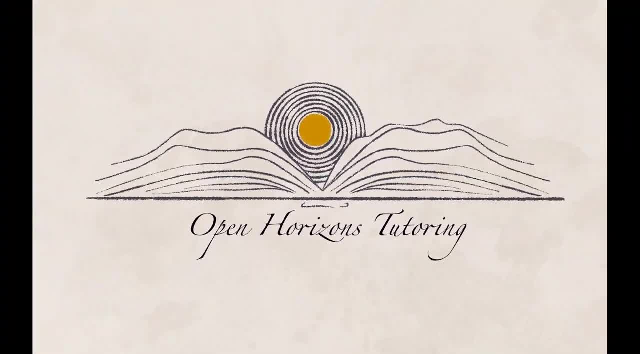 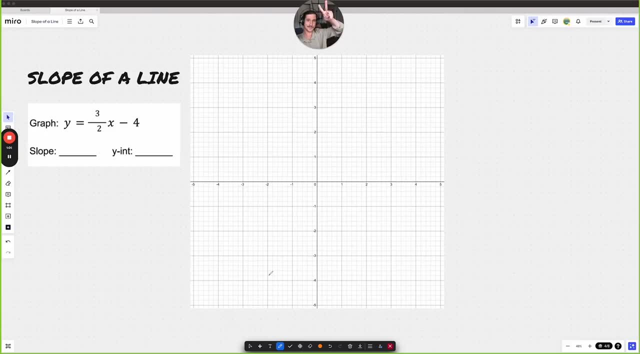 Hey students, welcome to Slope of a Line Today. let's take a look at the general equation: y equals mx plus b. So we would know that x is our input value, y is the output value we get out. So we want to take a look at m, which is your slope, and b, which is your. 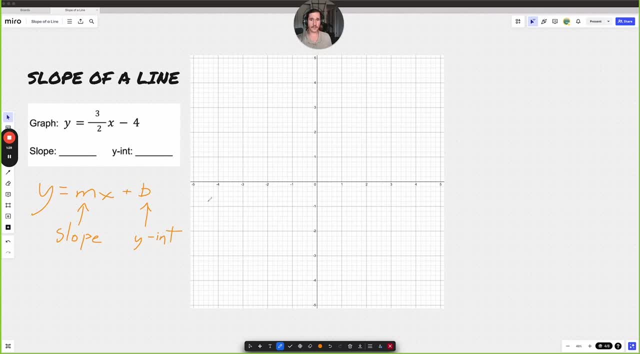 y-intercept. y-intercept is wherever it crosses your y-axis, that vertical axis, Say. the line crossed here, that would have a y-intercept or a b-value of 0.. If it crossed up here, that would have a y-intercept or b-value of 2.. 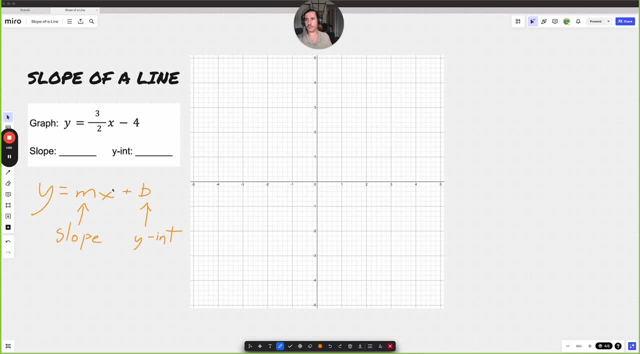 So we can find that using this general equation will help us to solve complex problems like this. So first let's take a look at our example problem. Our y-intercept will be found here. That is negative 4.. So y-intercept is negative 4.. Our slope is: whatever comes in front of your. 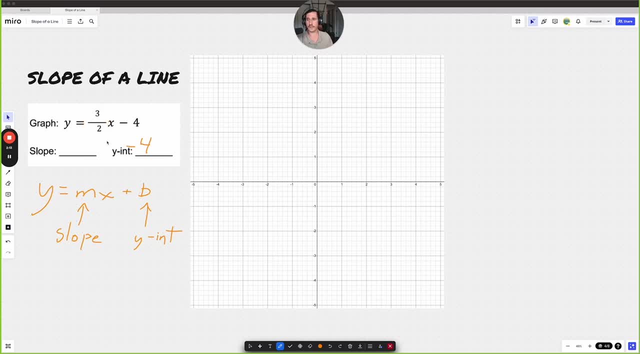 x-value, whatever that coefficient is. In this case that's 3 over 2.. Now, an easy way to think about how we graph this is starting with your y-intercept. If we were to plug in 0 for x, anything times 0, that's just 0. So, boom, that would cancel out all of this. 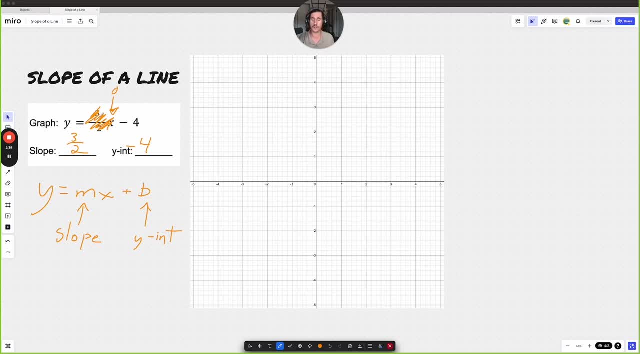 in front of your x and leave you with y equals negative 4.. So our first point- 0 comma negative 4, is something we can easily graph Boom right down there. Then we want to figure out where do we go from here. 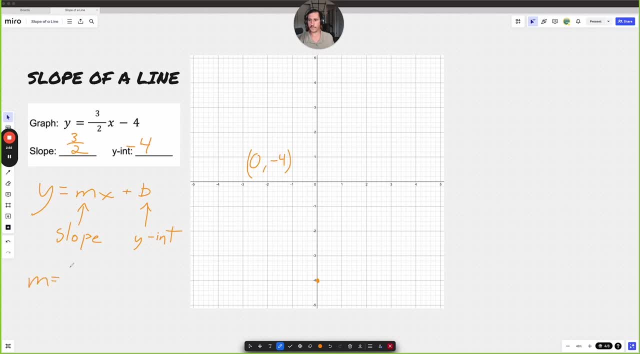 One way we can think about slope or your m-value is: rise how much it goes up over, run how much it goes over And by over. we always want to think when it's positive we're going over to the right. 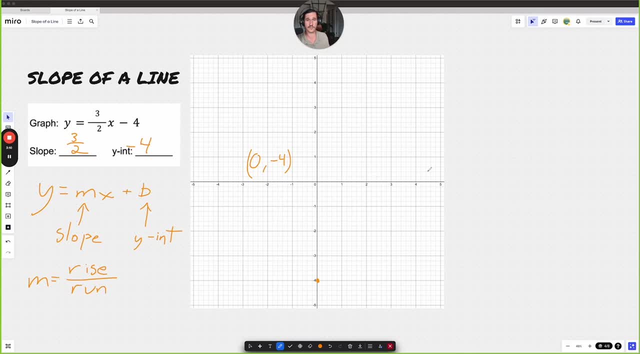 just like these numbers here are going in increasing order to the right, So rise, we're going to go up three: 1, 2, 3, over: 2, 1, 2.. For our next point HereThat is 2, negative. 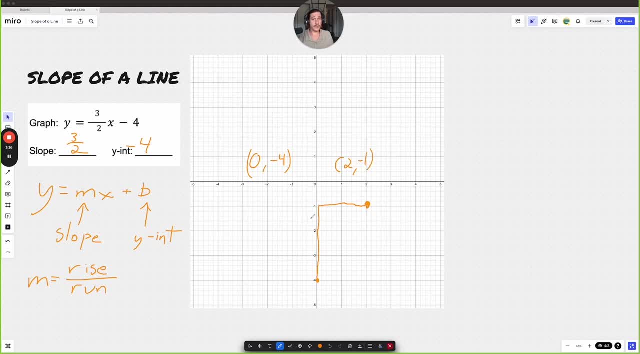 1.. All right, So we really only need two points to graph a line. So let's graph this thing, I don't know. There we go, All right. now let's do one thing: toGLUL assets, Something that counted out of it. here, There we go. Here's the next pointrect, Here's the next point, and then we're going to go over to 2, 1, 2, 3, over, 2, 1, 2.. For our next point here, that is 2 comma, negative, 00, negative 1.. All right, So we really only need two points to graph a line. So let's graph this thing. There we go, All. 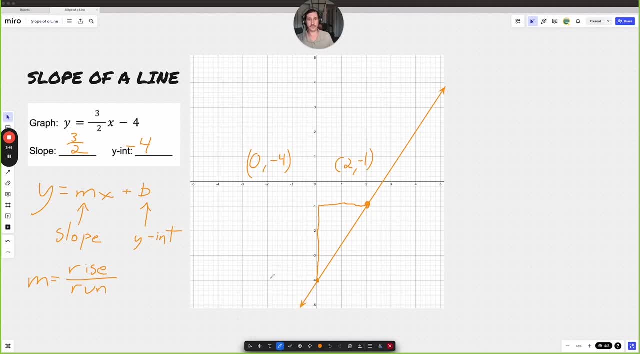 Now let's do one thing to double check. I always like doing gut checks just to make sure we've got it right. Is this line? let's move these a little bit- Is this line going to once again continue going up three over two? 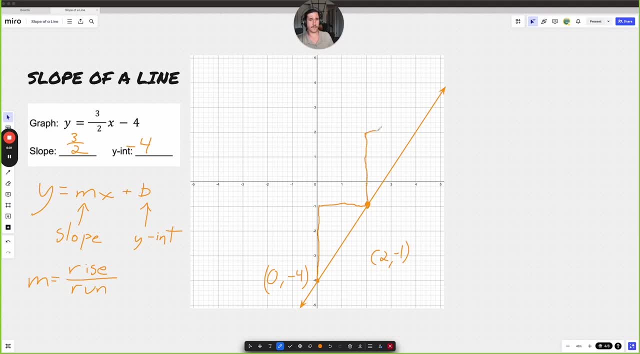 One, two, three up three. one, two over two. boom, It hits it again. That's how we can graph a line based on having its general equation. Let me know in the comments if you have any questions. Have a great day. See you next time.